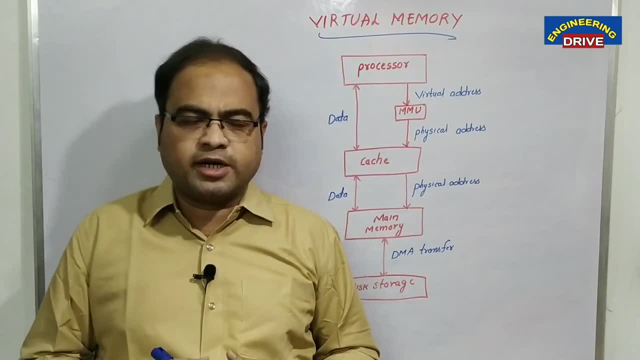 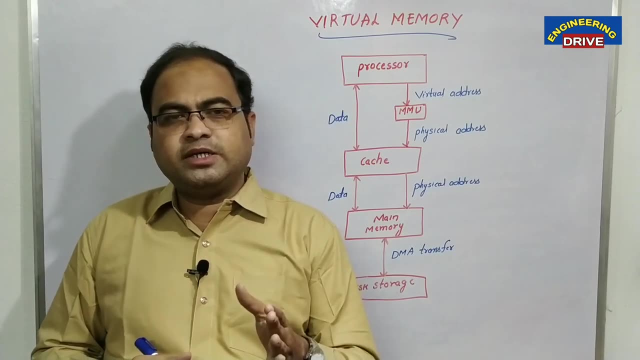 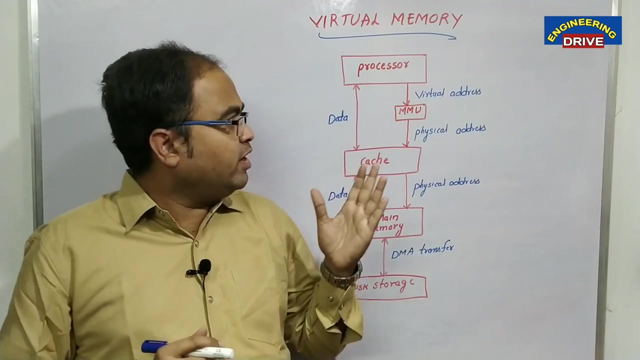 virtual here. first, Memory means a place to store the data in computer. What is the meaning of virtual memory? What is the meaning of virtual memory? You can simply use a word: duplicate which is not existent is virtual. Then why we are using this memory which is not existent in real? What is? 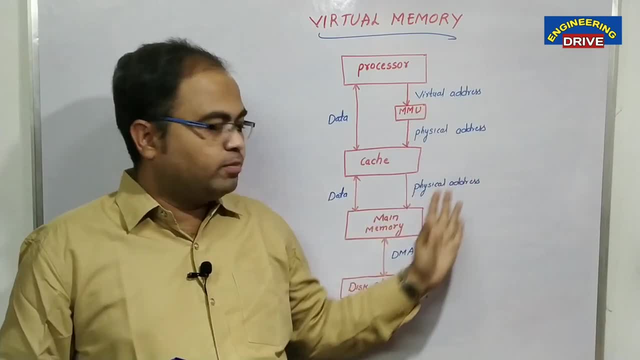 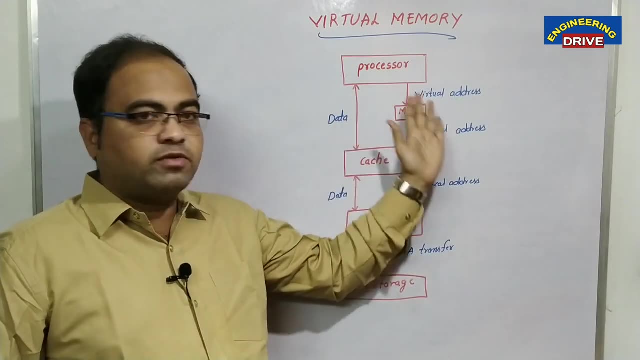 the reason behind this That I am going to explain you with the help of this diagram today in my video. My dear students, let us see here Everybody is having an awareness of this diagram. That processor will be there first, Then in between, cache memory, which is a small amount of. 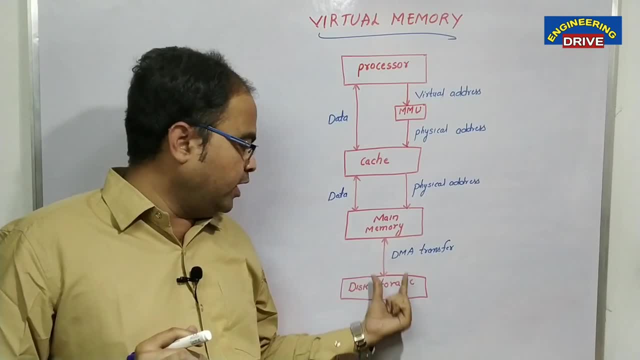 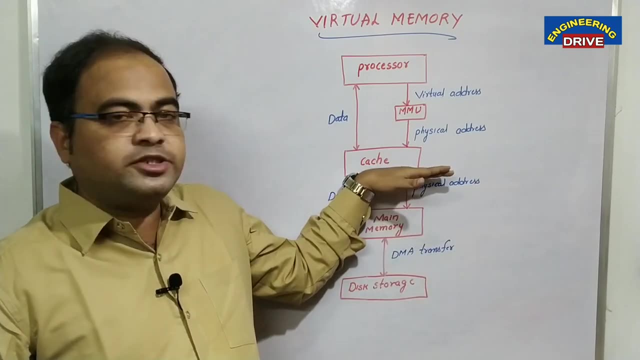 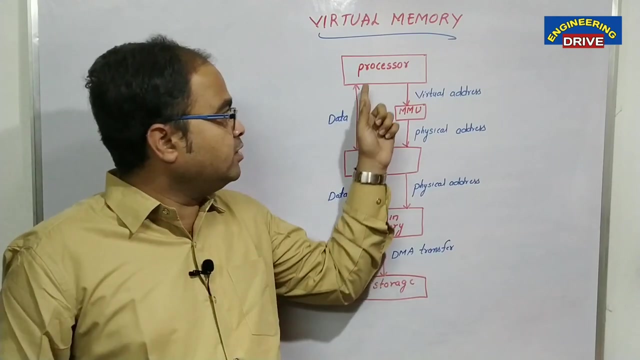 fast memory which is used in the computer. Then comes main memory And the last is our secondary memory. Secondary memory, main memory, cache memory, processor, So where the execution of the programs will take place, The execution of the programs will take place in processor, You know. 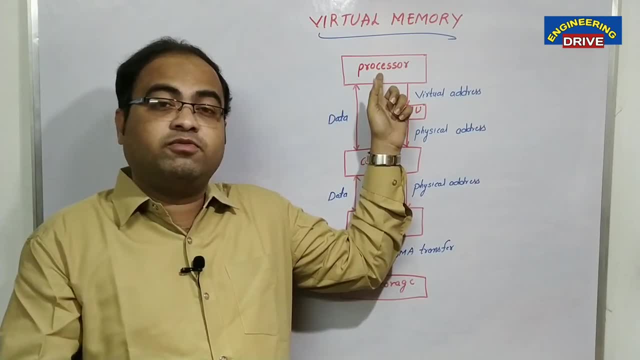 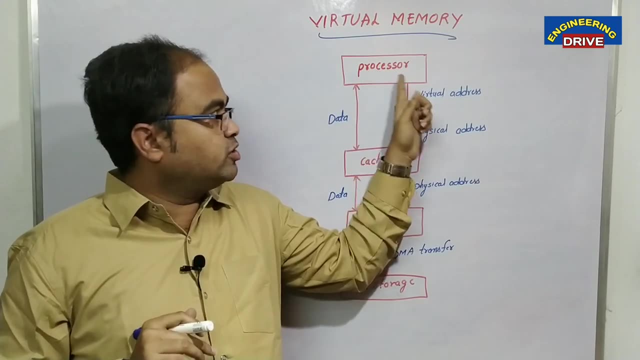 that. Where are the programs that users will use are stored? That is the next question. Execution will take place in processor. Where are the programs that users will use are stored? That is the next question. Execution will take place in processor. Where? what about the programs are? We will 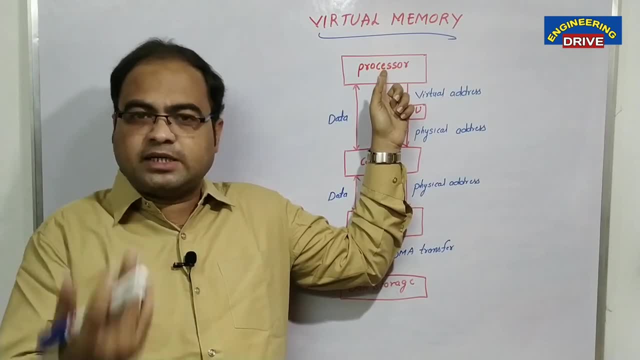 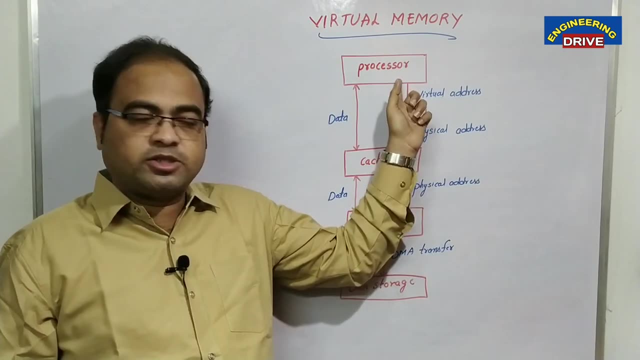 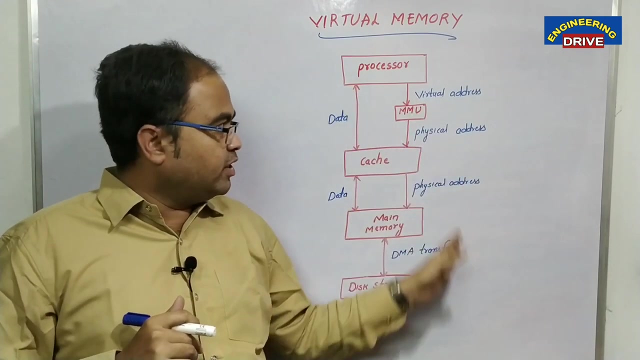 install programs in our computer. We will install some games. We will install some apps Where they are stored are in our computer, Secondary memory. Execution will take place in processor. Programs will be stored in secondary memory, That is, in disk storage. Now, always, our processor will not. 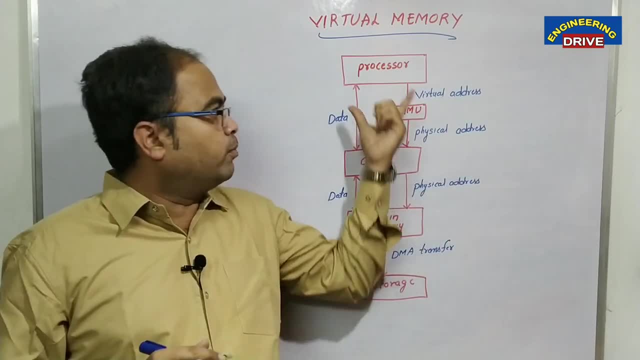 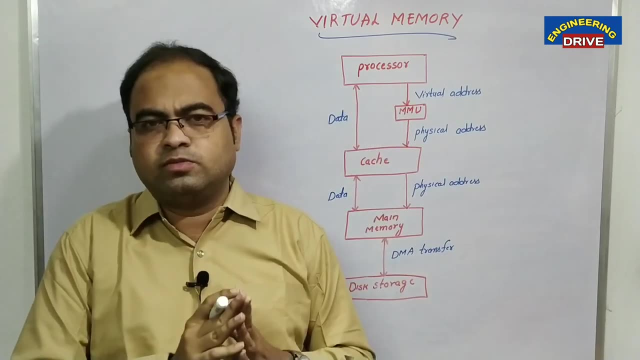 bring the data directly from secondary memory because processor speed is very fast- It is tremendous- Whereas the speed of secondary storage device is very fast. It is very fast, It is very slow. You know, if a fast processor wants to communicate with a slow secondary storage device, 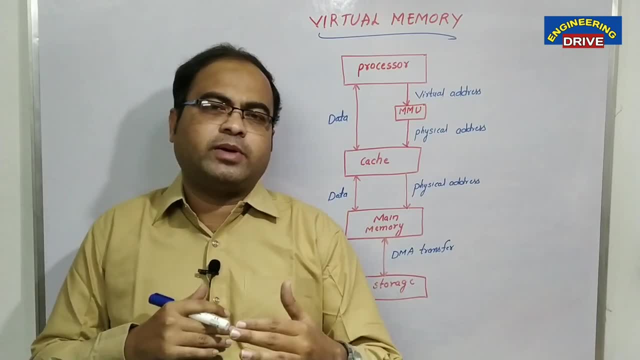 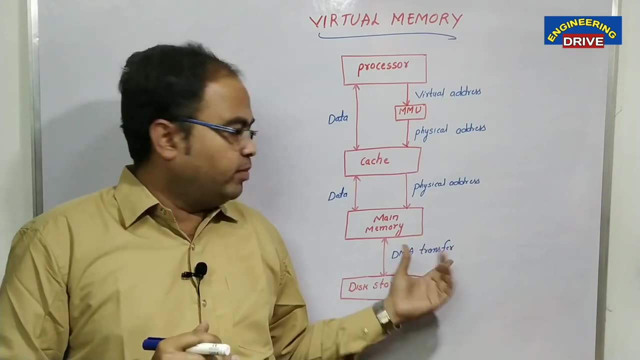 communication problem will come, Which means your computer may not be able to run as smooth as possible. OK, Up to now, it is clear. Now, to overcome this drawback, compulsory, a computer should make use of main memory. That's what we have learnt. Main memory is nothing but your. 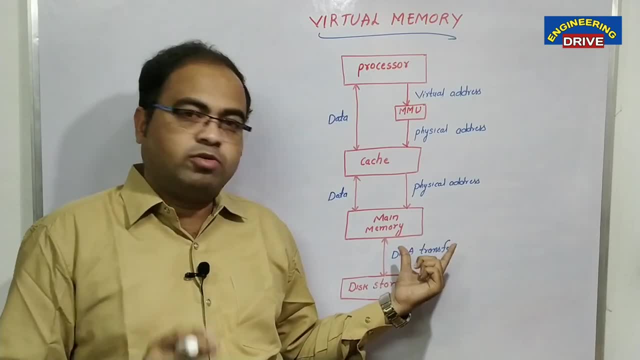 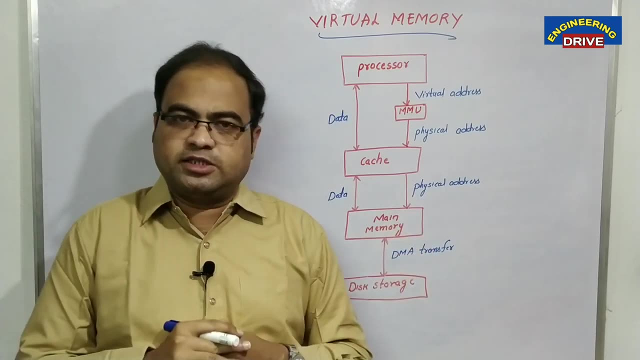 primary memory or random access memory. Now my next question to you: Whether the size of main memory is large or small, Whether the size of main memory is large or small, Whether the size of main is larger or the size of disk storage is larger, The answer is: size of disk storage is way larger. 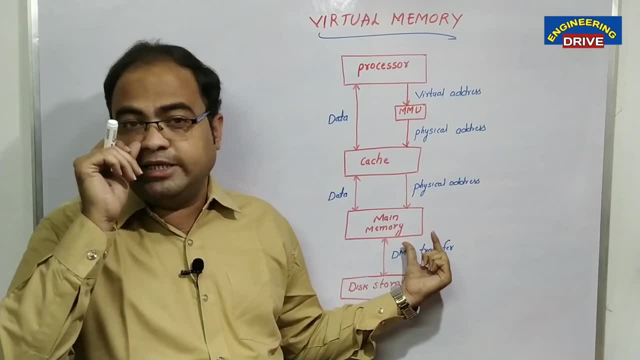 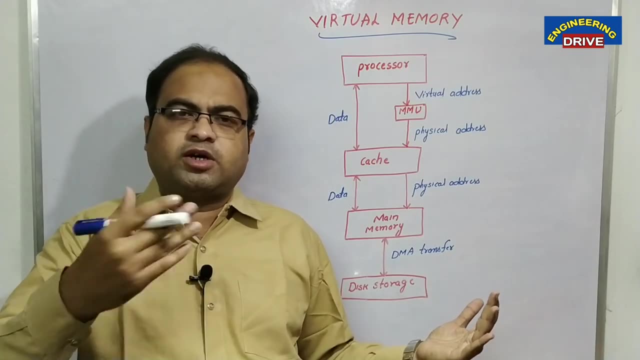 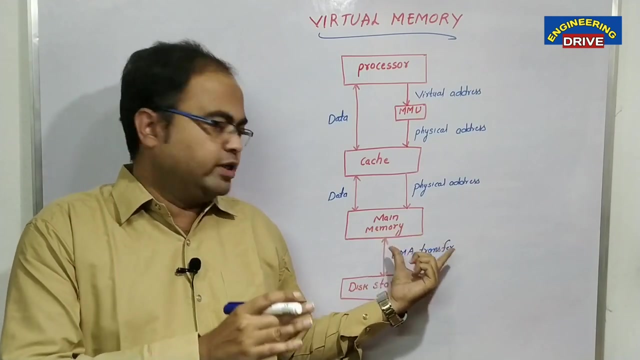 than the main memory. Generally, main memory nowadays comes in 8 GB, 4 GB or sometimes maximum 16 GB nowadays available. Okay, maybe it goes on increase day by day. that is secondary thing. Main memory size is. it is clear and cut point that it is smaller than secondary memory. 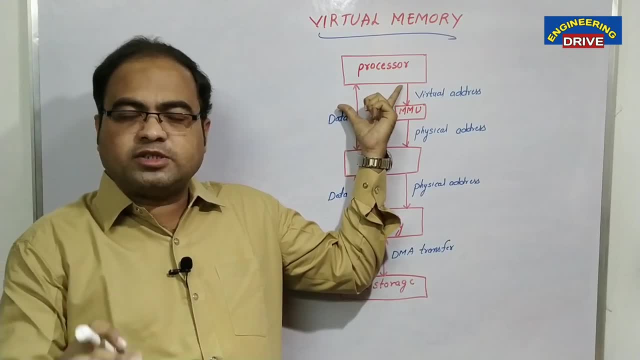 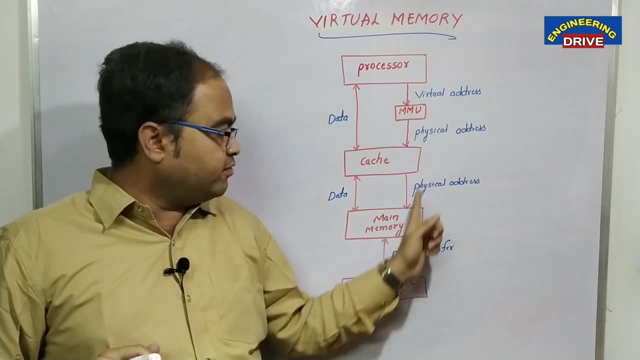 Yes or no? Now, processor: if a processor want to execute some program, what our processor will do? It will not take the directly from secondary memory. It will search the data first in main memory. If the data is not found in main memory, then processor will take the data from secondary. 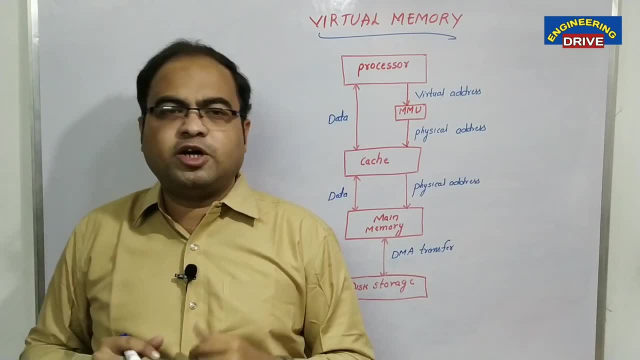 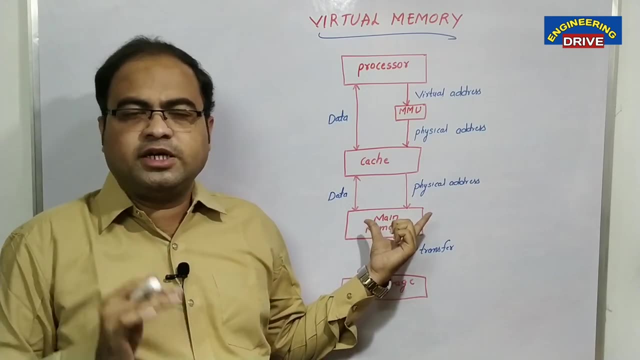 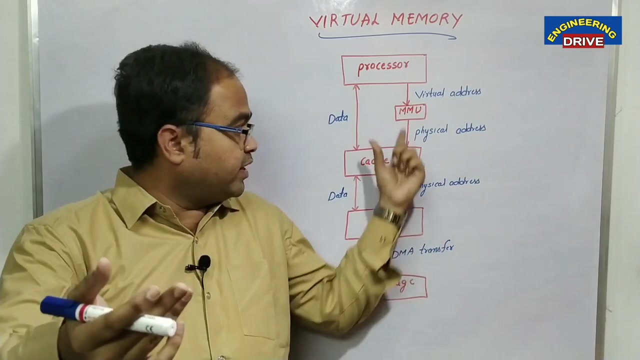 memory Now, in order to increase the speed of our computer, the point that we need to understand is: as much as data is possible in main memory, it is good for us, It is good for the speed of the computer. Okay Now, even if we want to increase the speed of the transfer rate between main memory and 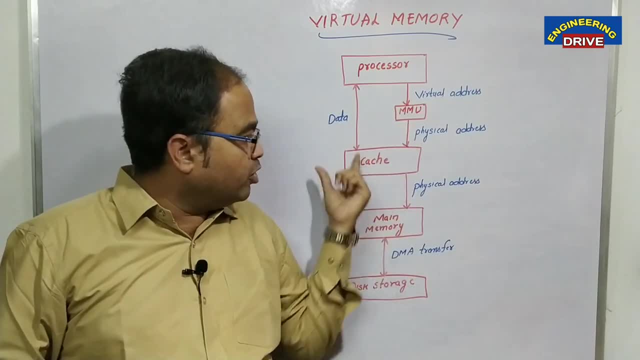 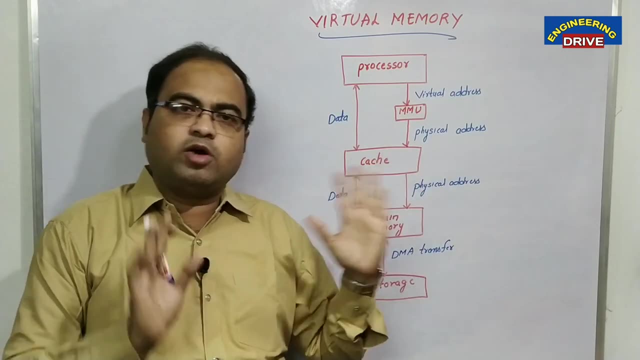 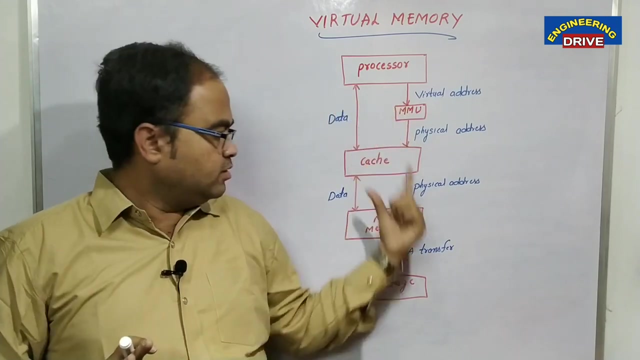 processor much more faster, then we can make use of cache memory also. Cache memory is a small amount of fast memory. That is what in memory hierarchy we have discussed. Okay, If processor want to, in simple terms, I will explain to you what about the sizes are. Secondary memory size is very large. Main memory size is lesser than secondary memory. Cache memory size is much more smaller than main memory And the size of the processor is also much more smaller than cache memory. That you need to understand, Okay, But when coming to the speed, processor is the fastest one, Cache memory is the second fastest Main. 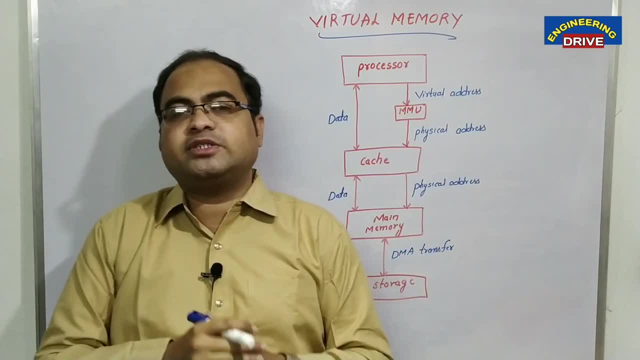 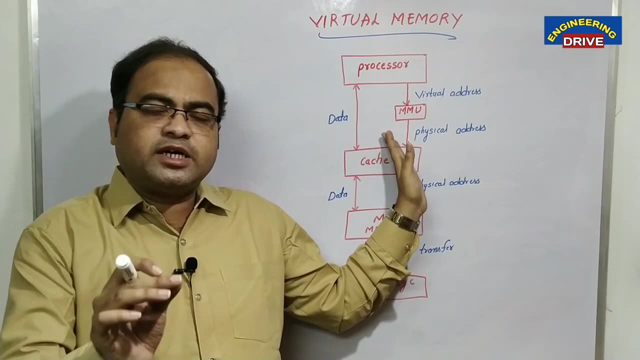 memory is the third fastest And the slowest one is our disk storage secondary memory. Okay, Clear Now. if our processor needs some data, it will search the data first. Now you tell me, according to the diagram, It will search in cache. 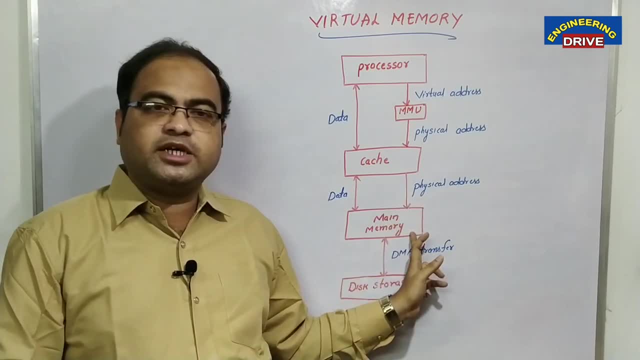 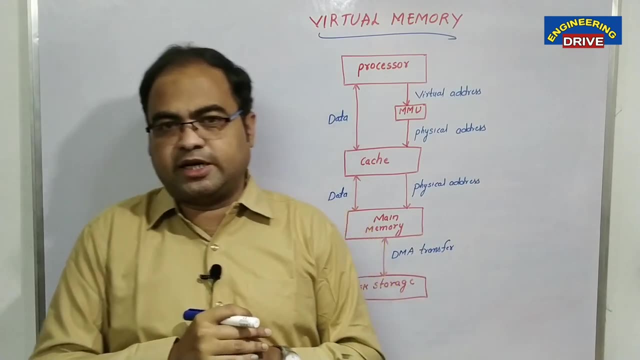 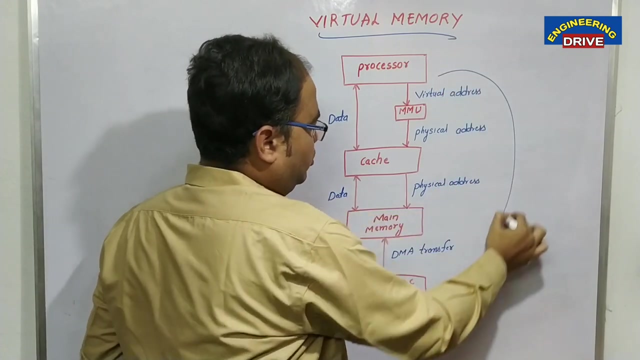 memory first. If the data is not found in the cache memory, it will stay check in main memory. If it is not found in main memory, then last preference will be given to secondary memory to search the data. If processor every time will take the data from itself to disk storage means, it will be a very 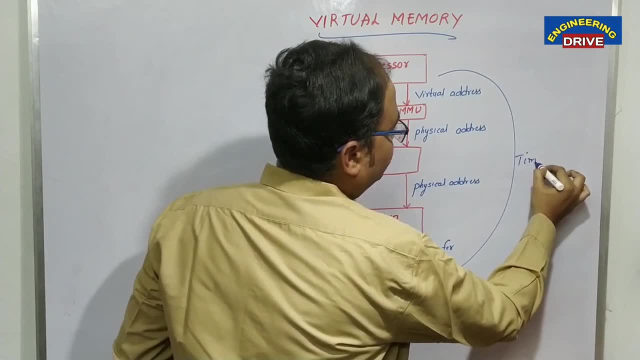 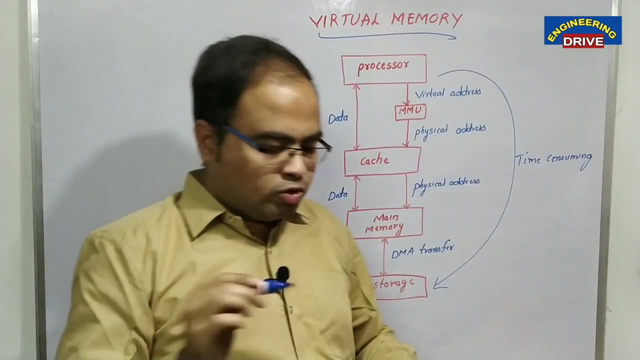 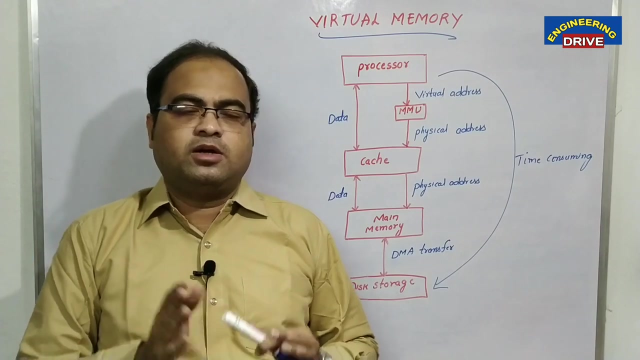 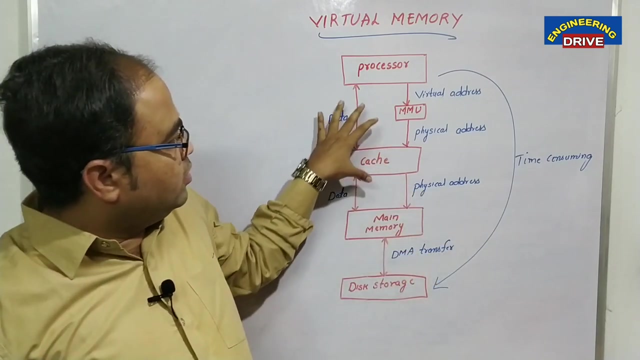 time consuming process. Okay, It is a very time consuming process. So, finally, we want to increase the speed of our computer now. Now, what our computer will do means what is the technique that our processor will do? is means processor. let us say, in our concept, if processor want to access the data, it will check. 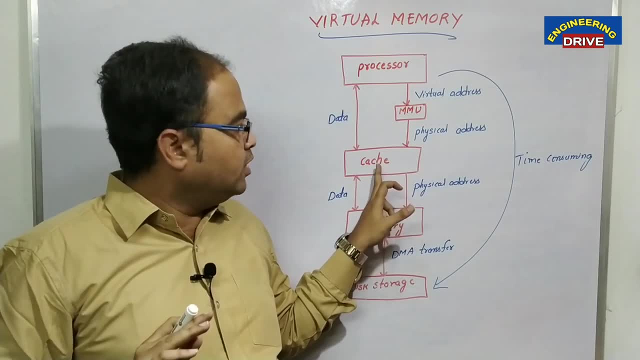 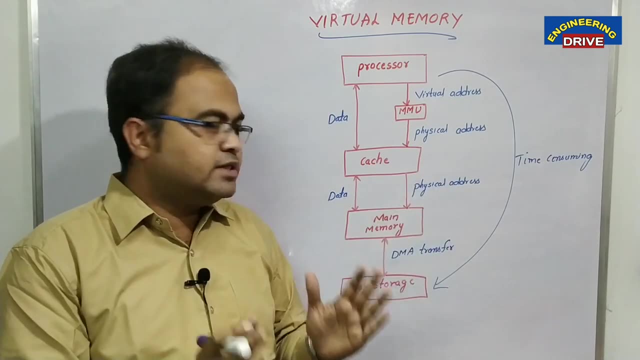 in cache memory first. If the required data is found, no problem. Next, it will check the data in main memory. If the required data is found, no problem, Program will be executed. So if the required data is found, no problem, Program will be executed. Now sometimes what happened? it is clear. 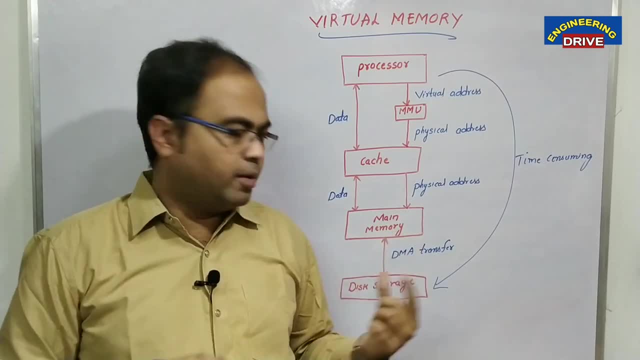 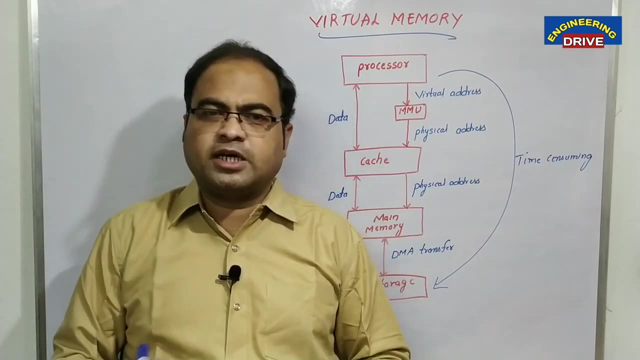 and cut point that the size of the main memory is very small compared to the size of the secondary memory, So our main memory can't able to store more number of programs at a time. Yes or no? It is a clear and cut point. Everyone will agree with this. Now, sometimes, what we want, we want to increase. 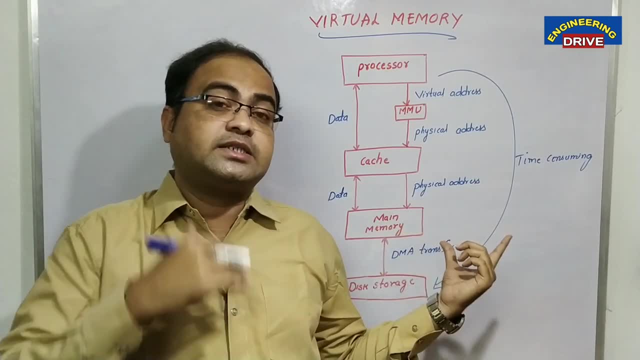 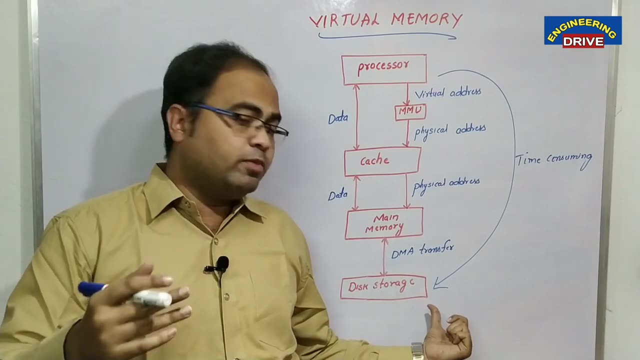 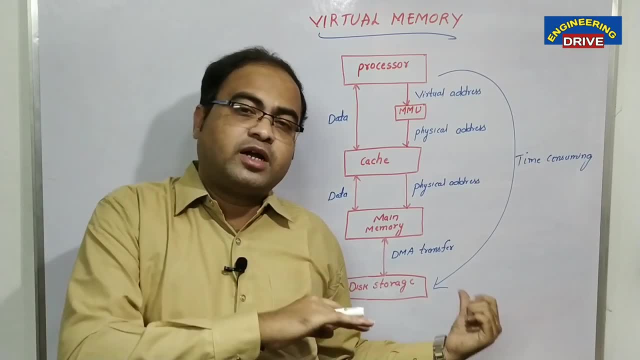 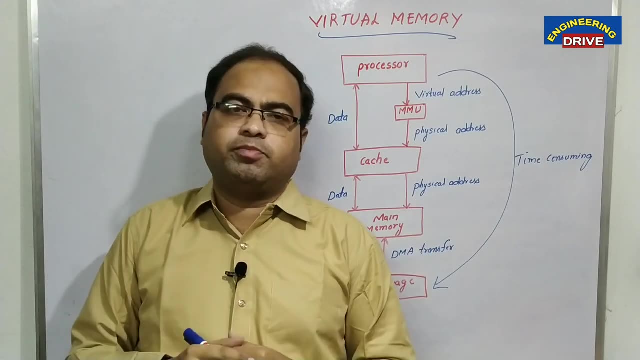 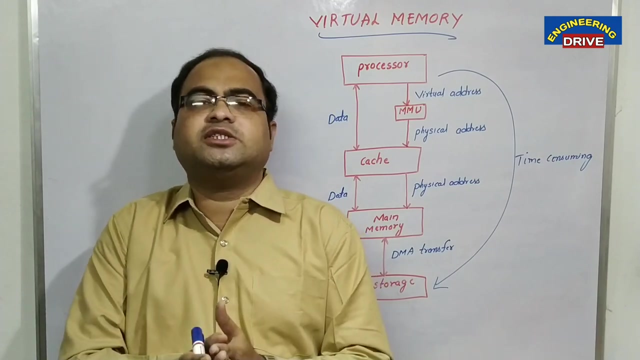 Secondary memory is 1TB, 2TB sizes became, sir, why we are unable to get the size of main memory further. The answer to your question is: main memory is very, very costly to implement. Okay, So our computer manufacturers. they can able to manage a size of 8GB or 16GB up to a maximum. 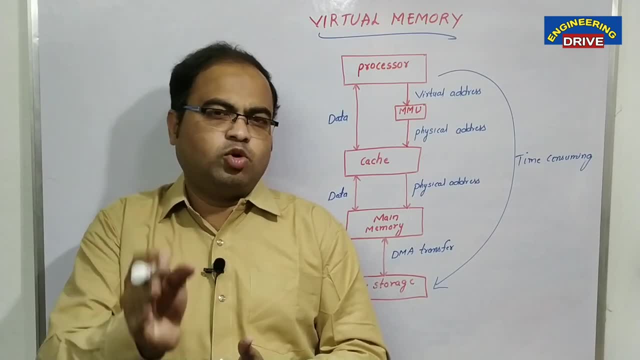 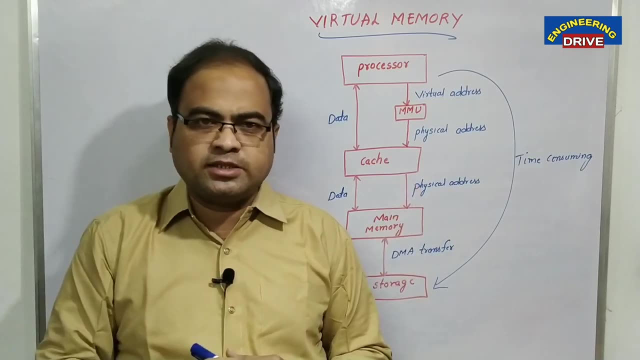 extent now. Okay, So now you want one technique now to increase the size of main memory. One option is you need to purchase the main memory of higher size, but it is impossible, So you need to purchase the main memory of higher size. 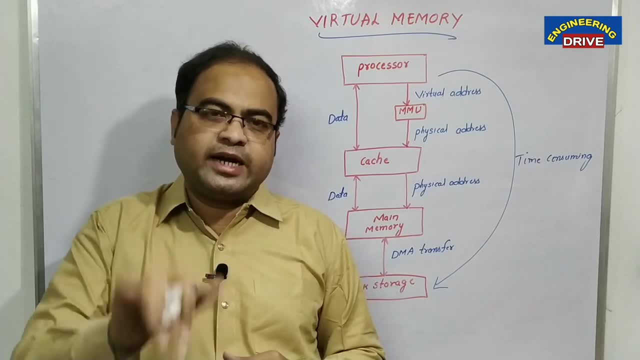 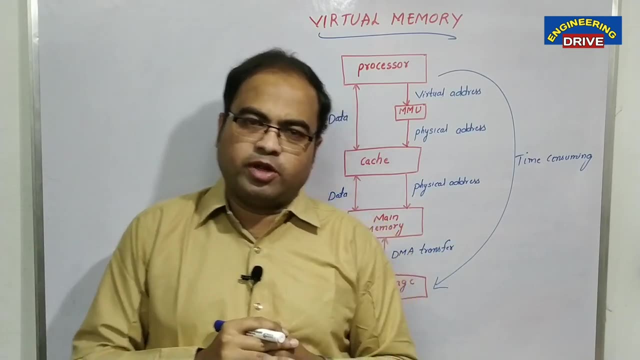 It is a very costly approach, So you cannot do that. Second option, sir: what is the second option? I want to increase the size of my main memory. now, If you want to increase the size of your main memory, what you need to do is take some space from secondary memory. 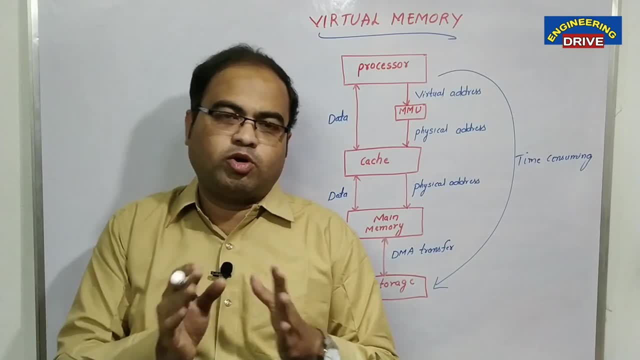 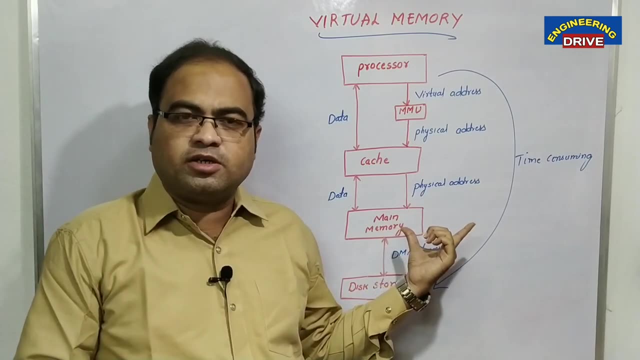 and treat it as a main memory. Hope you got the point. In simple words I am explaining to you. first, If the size of main memory is not sufficient to execute more number of programs, if it cannot store more number of programs, then 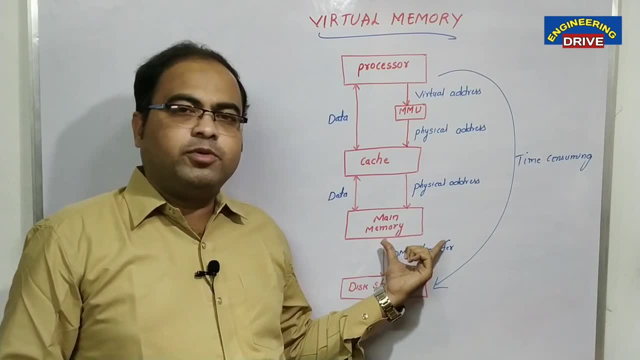 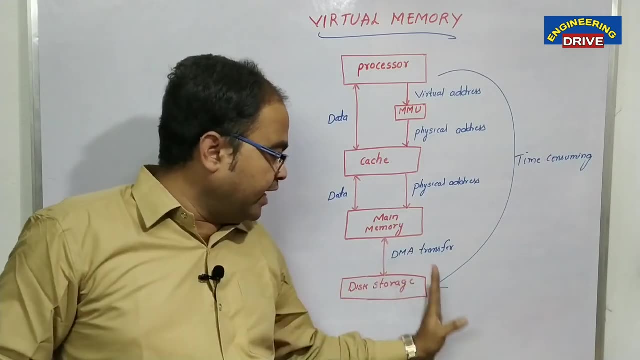 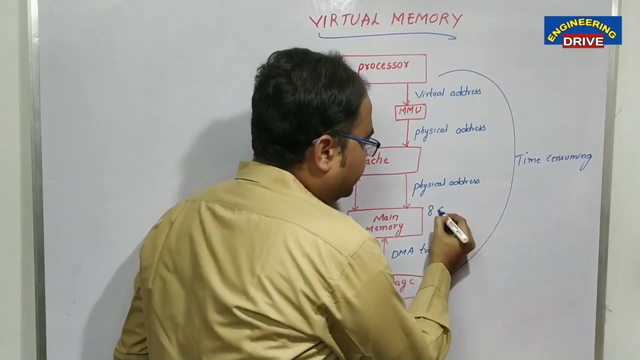 what we can do is we can use one approach. One alternative approach is our computer can make use of secondary storage or disk storage as a main memory. I am not saying that entire disk storage should be used as a main memory. some part of the disk storage, Let us say our main memory size is 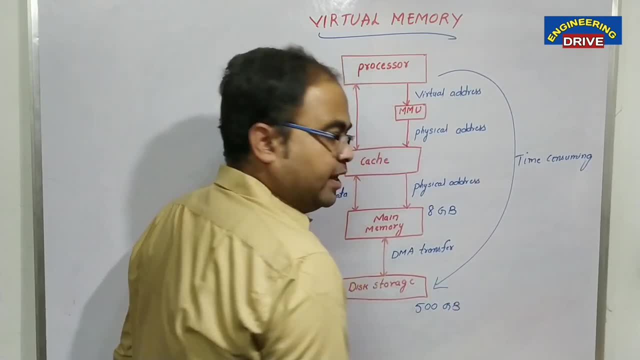 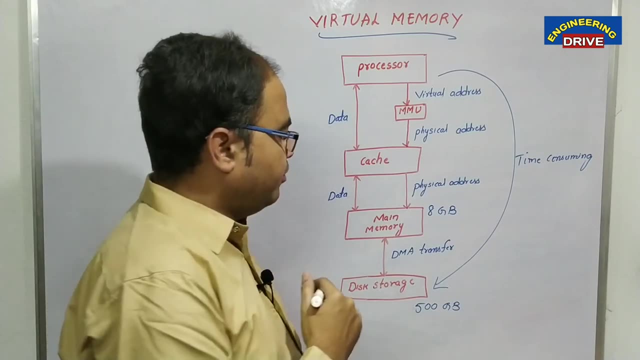 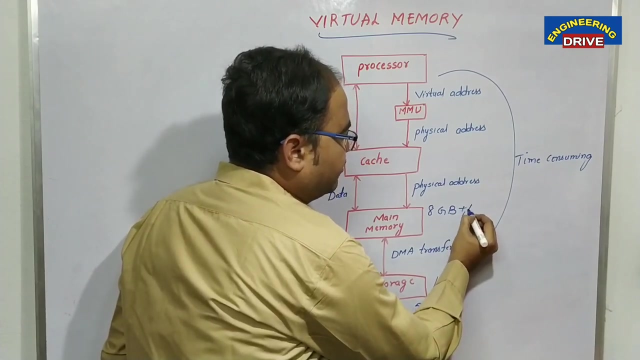 8GB and our disk storage size is, let us say, 500GB, Then what we can do is we can use one for me now. so what our computer can do: miss out of 500 GB, it can take from here extra 4 GB that. 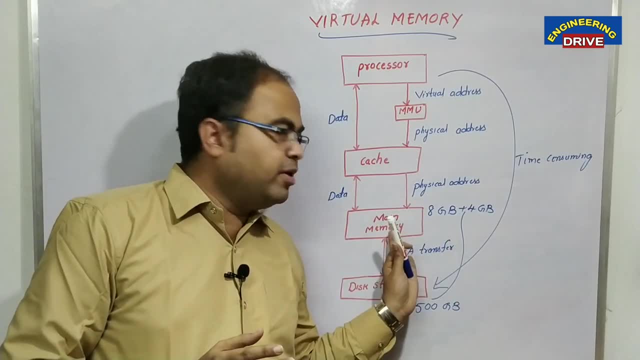 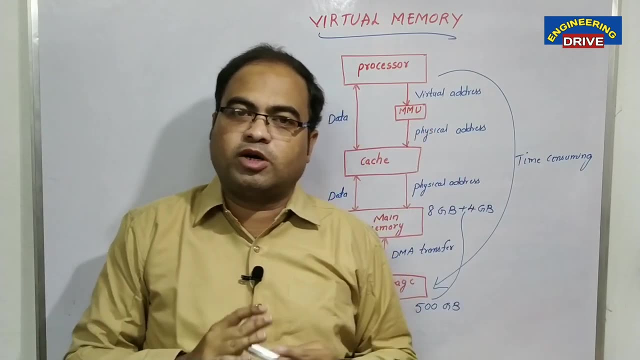 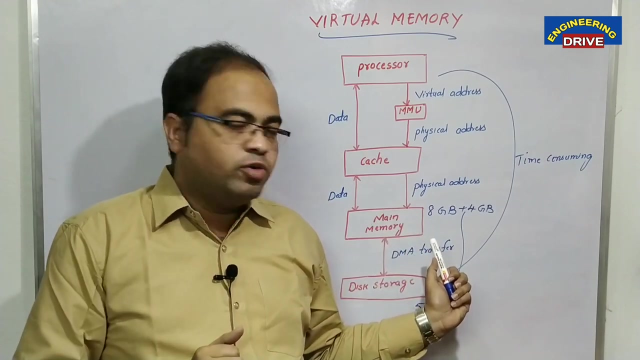 extra 4 GB is nothing but an extra main memory that is added now here. now, this extra 4 GB will become your virtual memory. hope you got the point. okay, actually, this 4 GB is not a main memory in reality, but what we are doing here, this 4 GB we are taking from secondary memory, yes or no, and we 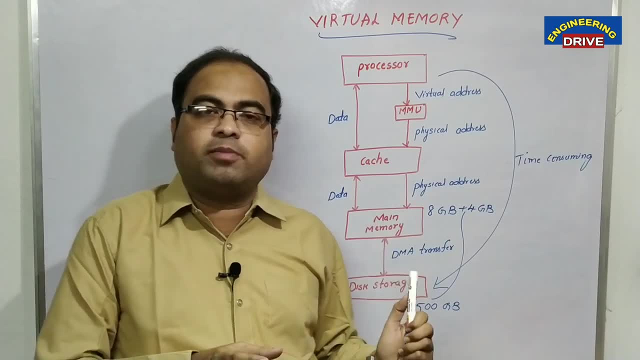 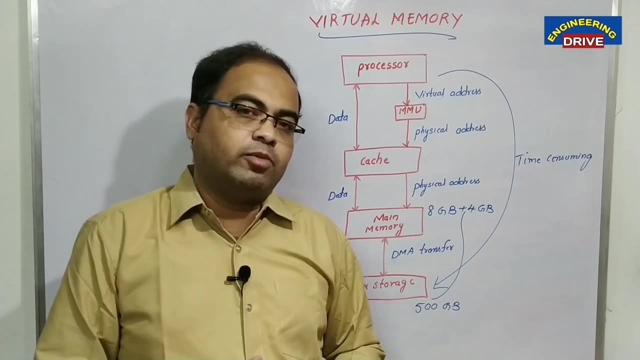 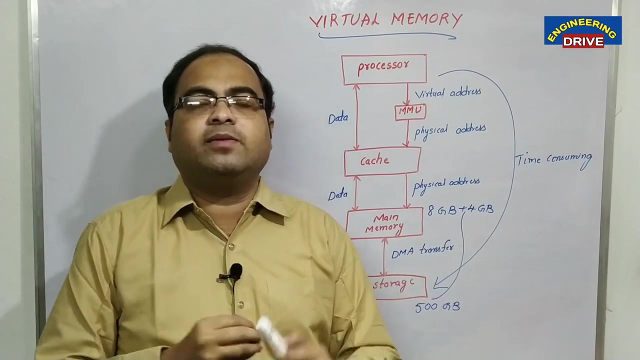 are using it as a main memory. that's why we call this topic as virtual memory, because it is not really present, but virtually we are making it as a main memory. so what is the advantage we will get here? the advantage we will get here is we can increase the size of the main memory and it can. 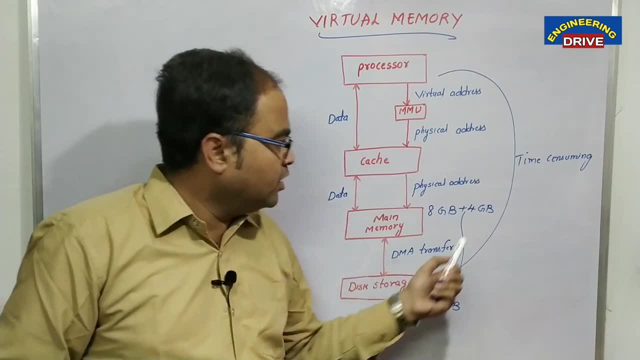 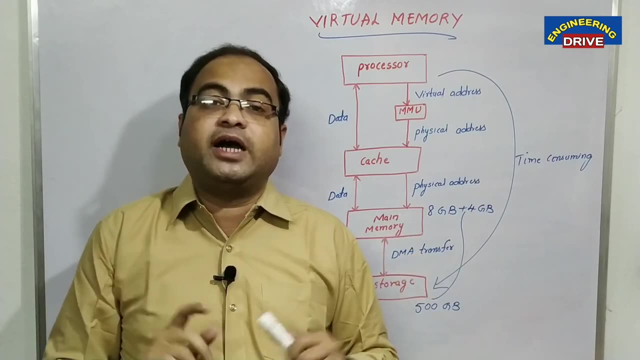 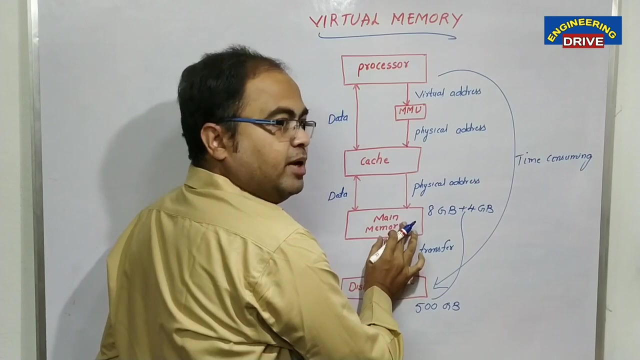 able to store more number of programs. now the next question, sir: this 4 GB. how this 4 GB will be removed here and it will be added in main memory. it will not be added, my dear students, automatically. this 4 GB will be used by our processor as if it is a main memory. how this? 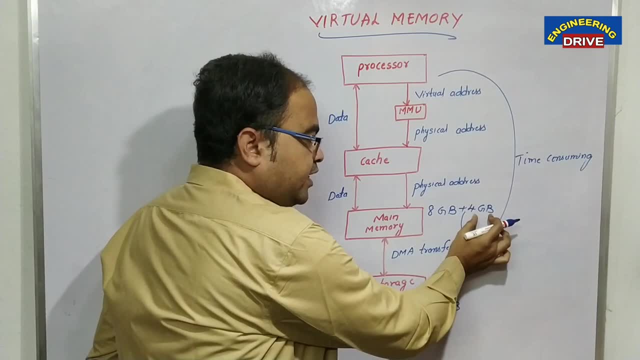 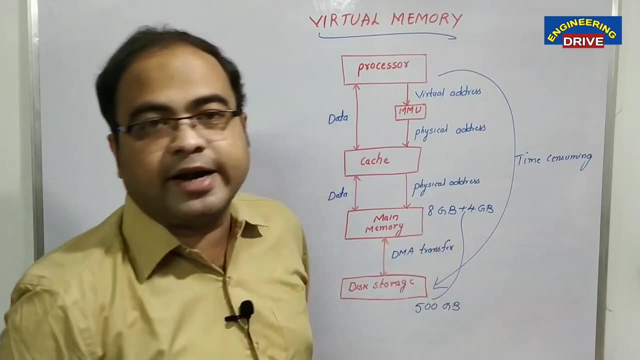 data transfer will take place from main memory and disk storage. how the data transfer will take place between this 4 GB and the 8 GB of memory with the help of one technique known as DMA transfer. we call this topic as direct memory transfer. what is direct memory transfer? 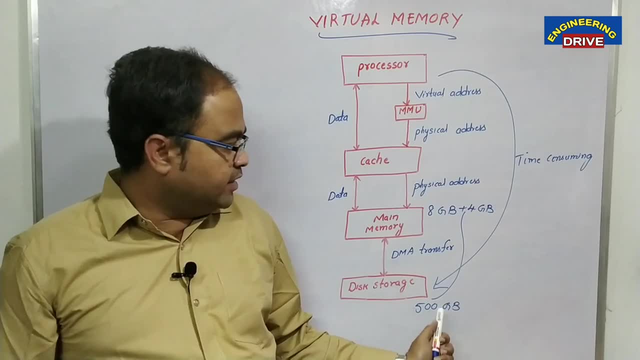 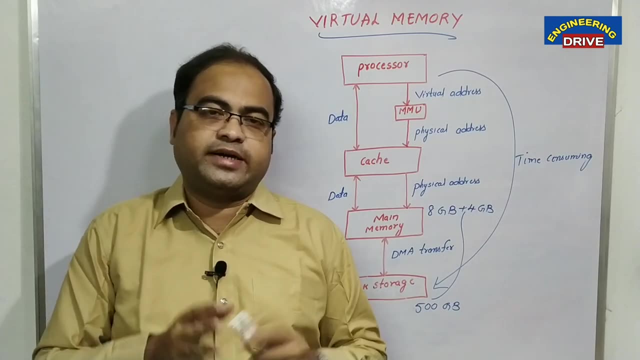 we are using some part of disk storage as a main memory. from that the data will be transferred to main memory. we call this concept as DMA, direct memory access transfer. okay, direct memory access. I will prepare one separate video to you how this DMA will work, how the access day, how the data will. 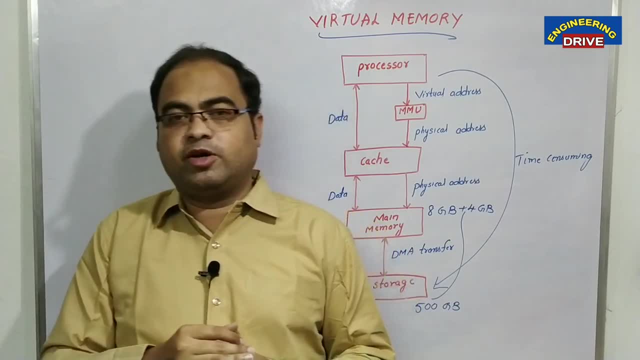 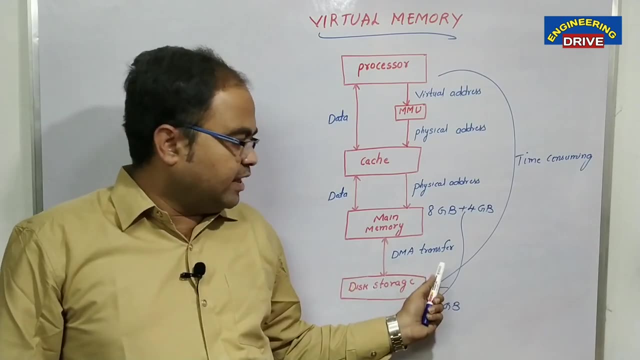 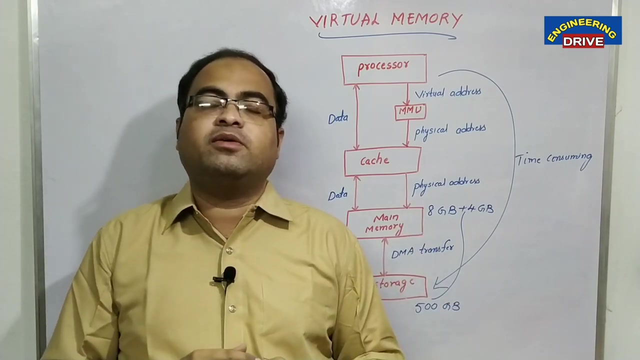 be accessed from secondary storage devices to directly main memory. everything I am going to explain with the help of separate video on the direct memory access, but now you just remember this point. thus, extra memory that can be used from secondary memory in terms of main memory is known as the memory virtual memory concept. 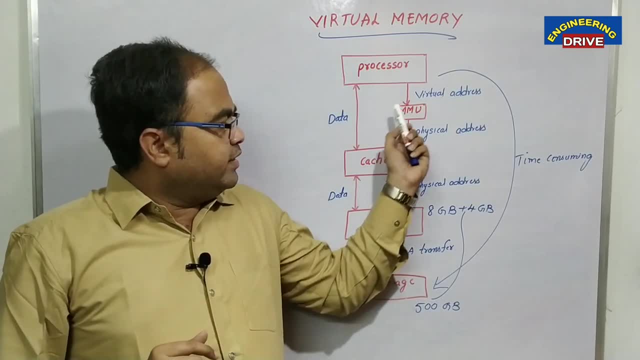 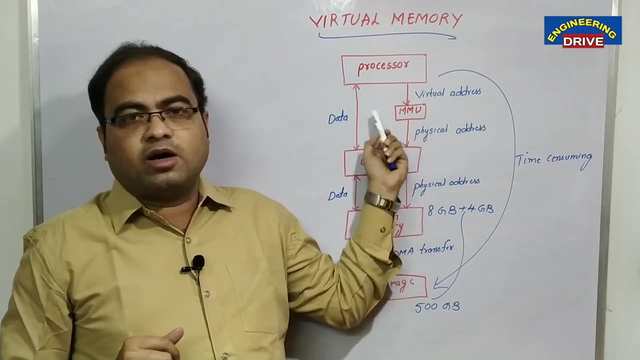 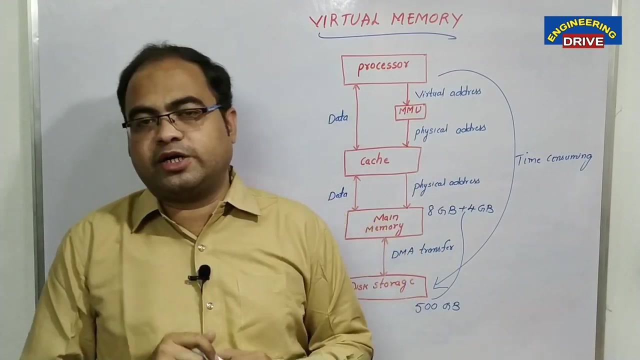 okay, hopefully it has been clear to you now directly to implement this virtual memory technique. what our computer will do means it will come. it will have one more hardware unit in in the system. the name of the hardware unit is MMU- memory management unit. what is the name of? 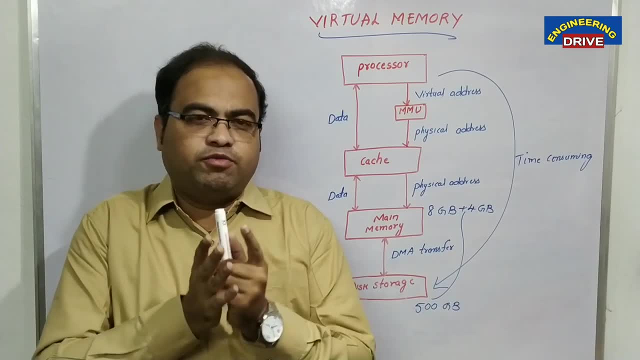 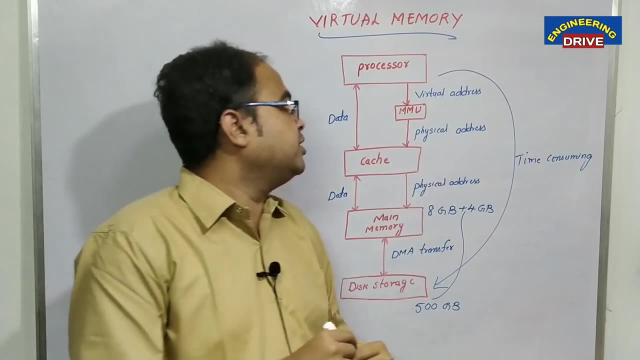 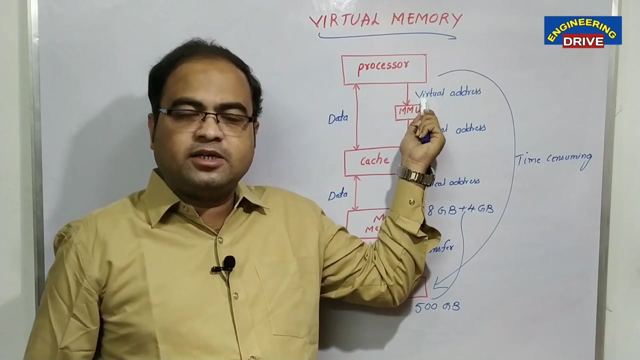 this unit, whether it is a software or it is a hardware, hardware everything. whatever we are going to discuss in our CO subject is mostly hardware memory management unit, what this memory management unit will do suppose. if our processor want to access the data of our virtual memory, then processor will send one address which is a virtual address. this virtual address will be: 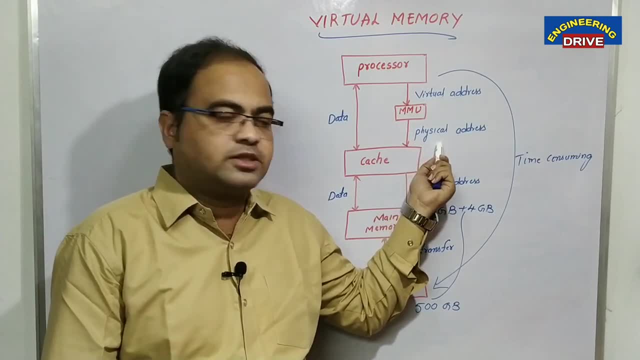 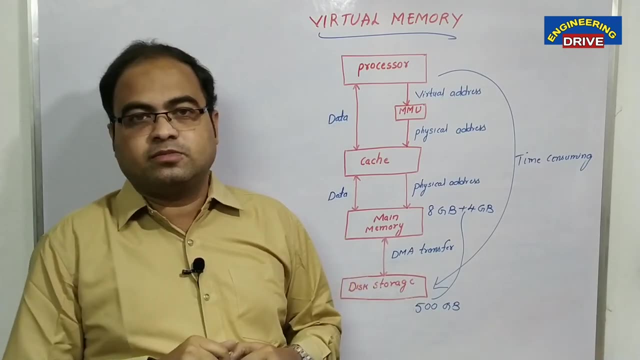 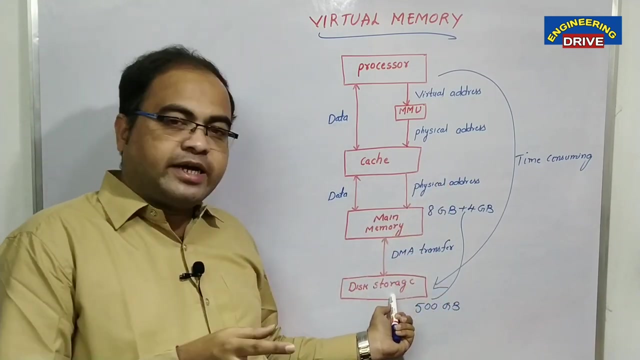 translated by our memory management unit into a actual physical address. through this physical address, the required data from secondary memory, which is assumed as main memory, will be accessed. okay now, once that physical address will be passed to the secondary storage device, what happened? this secondary storage device will. 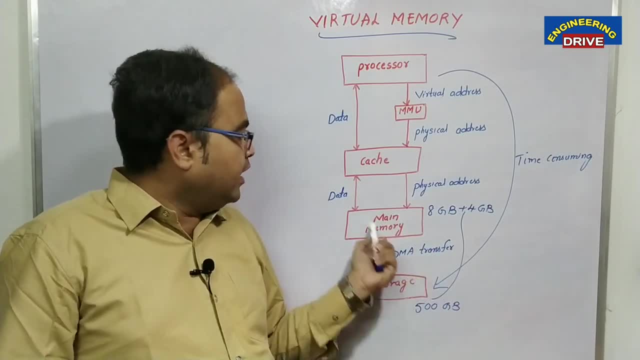 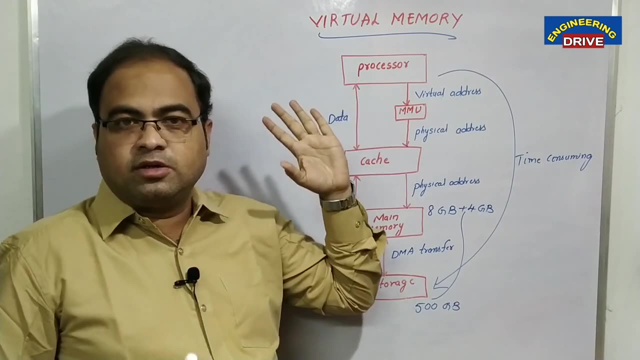 communicate with the main memory with the help of a DMA transfer method and the data will be communicated to the processor. you can see here: main memory to cache, cache to processor. second time, when the processor will request the data, processor won't search the data in main memory. 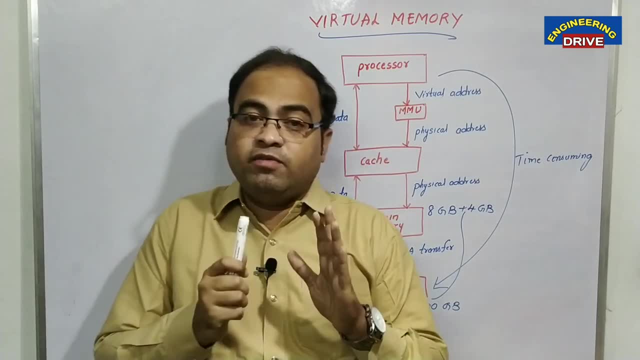 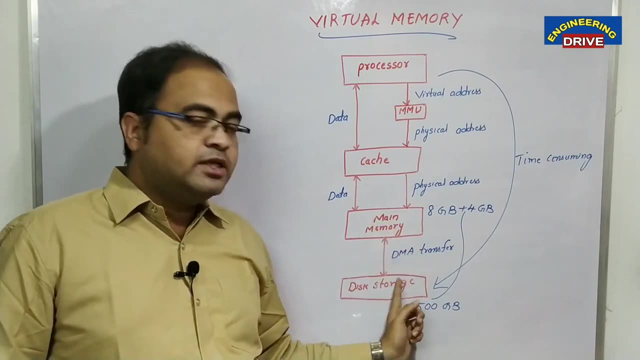 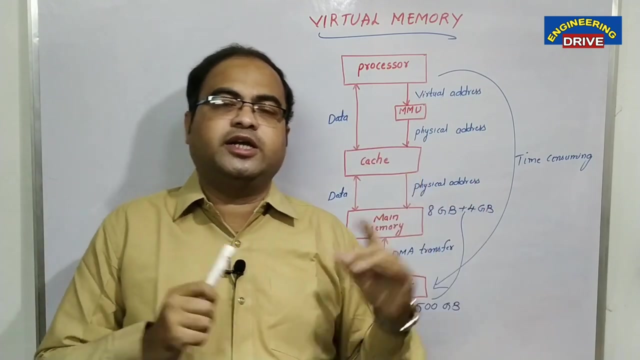 processor will search the data directly from cache memory. if the data is not found in the cache memory, then only it will search in main memory. if it is not found in main memory, then it will search in. finally, secondary storage device, that is, disk storage. okay, hopefully the concept of virtual memory has been clear to you, sir, when we need to. 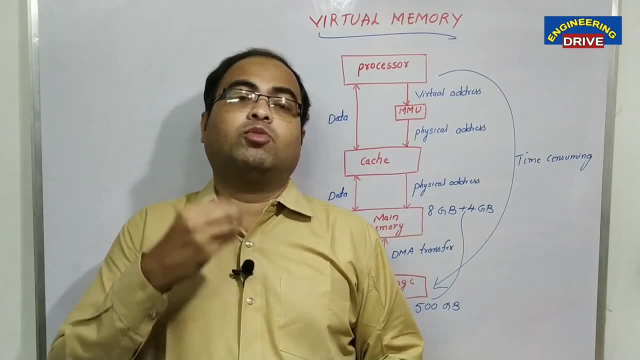 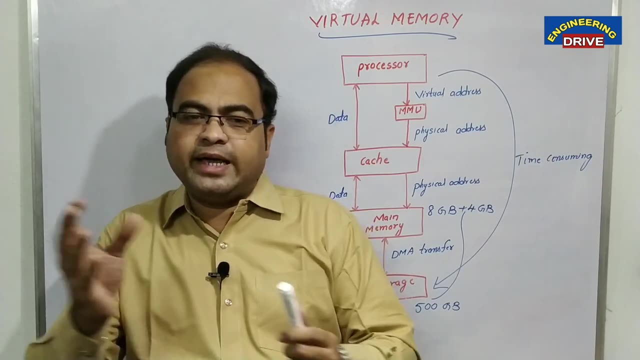 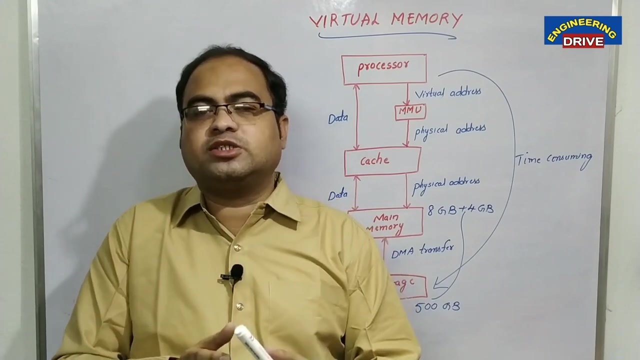 use this virtual memory if your main memory cannot able to store more much amount of data. if you want to increase the size of your main memory, then one alternative method is you can take some space of secondary memory store, secondary storage device and you can use it as a main memory. we call this. 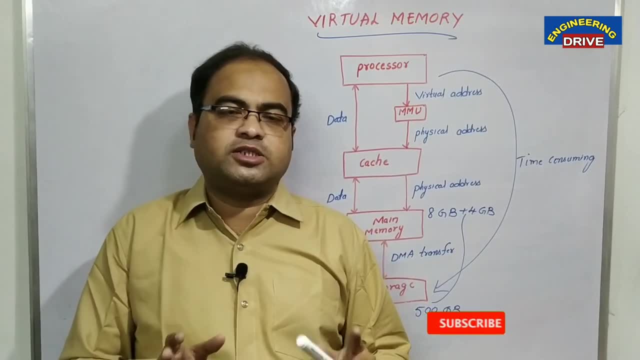 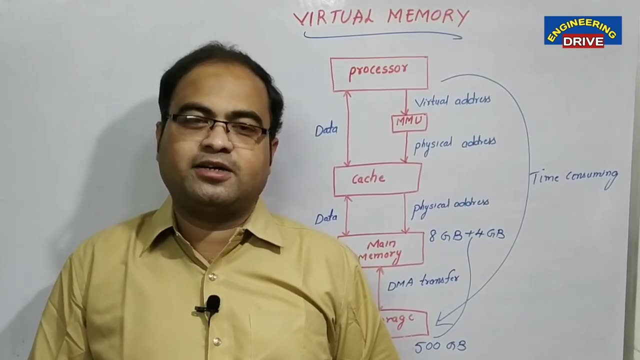 concept as virtual memory technique. okay, hopefully the concept of virtual memory has been clear to you. with this, let me close my today's session of video. see you soon, everybody. take care, Allah Hafiz.